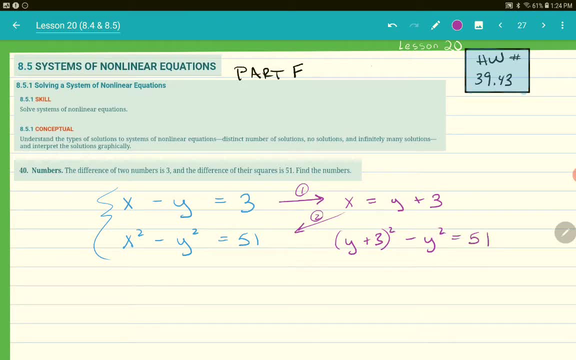 So now I have a single equation with one variable and I can solve for y. So foiling out the y plus 3, I get y squared plus 3y plus 3y, which will give me 6y plus 9 minus y squared equals 51.. 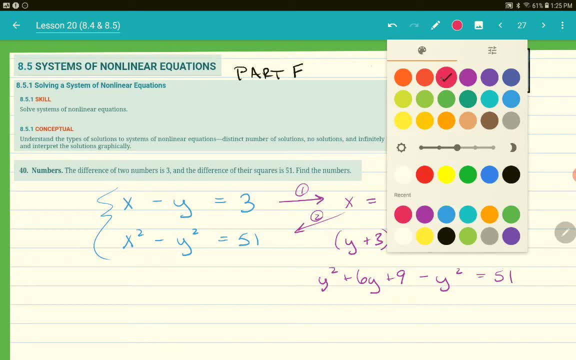 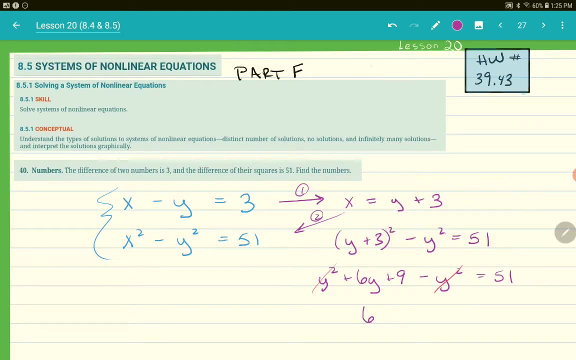 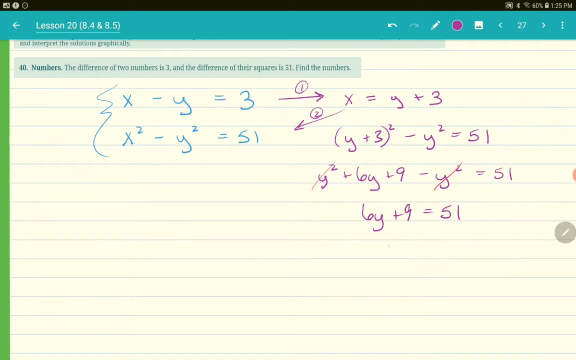 My y squareds cancel. I have positive and a negative y squared which gives me 6y plus 9 equals 51, which gives me, subtracting 9 from both sides, I get 6y equals 42. And then y equals 9.. 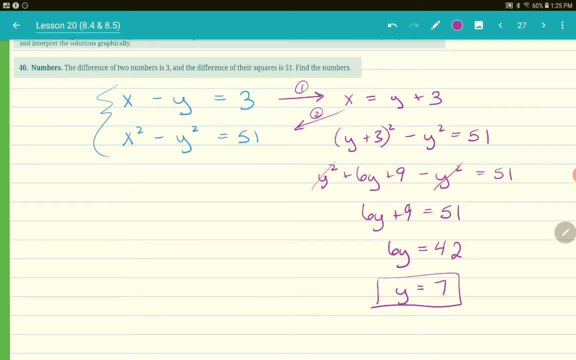 So I have a solution for y. Now to find x, I just take my x and plug that into the first equation. So I already solved for x in that first equation. so that gives me. you know, what I'll do is a different color. 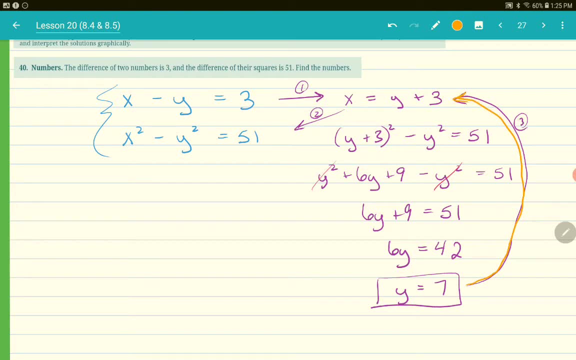 Oh, some color coding here. So my third step will be to plug in the 7 into this equation. So I know now. I now know that y equals 7.. So x must be 10.. So my solution is the ordered pair: x equals 10 and y equals 7.. 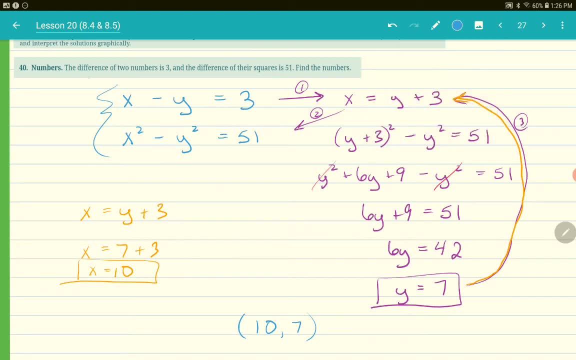 And I can always check that. so, looking at the original wording, the difference of two numbers is 3.. Is the difference between 10 and 7 3?? Yes, it is, So that satisfies that. And then the difference of their squares is 51.. 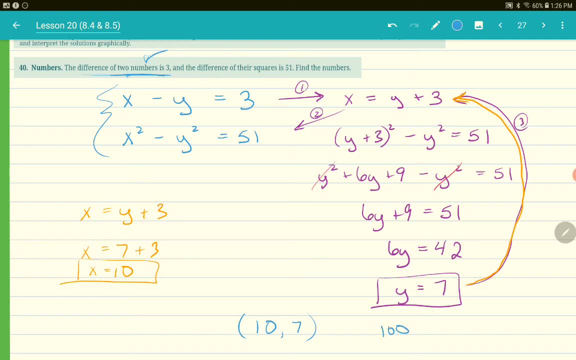 So is the difference of their squares 51?? Let's see 100, 10 squared is 100, 7 squared is 49, and that does equal 51. So that is checked, So that is confirmed and is my solution.